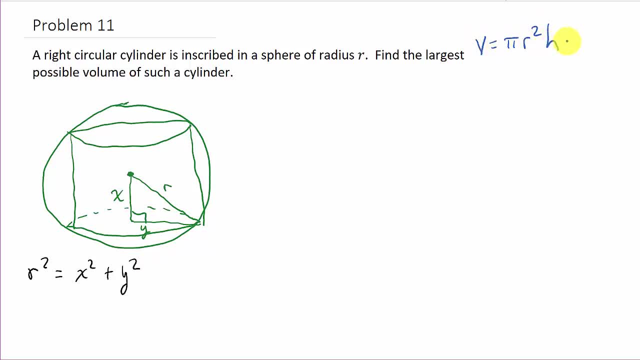 The volume is pi r squared times h- It's the area of the bottom- times the height. Okay. So in the problem we have here, the volume is going to be pi times okay, y squared. Okay, It's the area of the bottom. 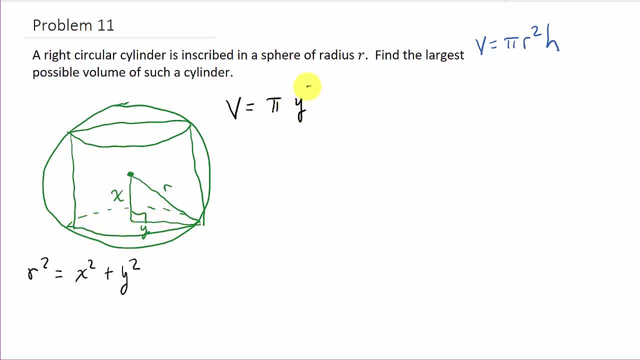 Okay, And that's going to be y squared times the height. Okay, Let me just draw a picture real quick over here of a cylinder. That's r and that's h, And it's pi times r squared times h. Okay, So we've got pi times this y squared. 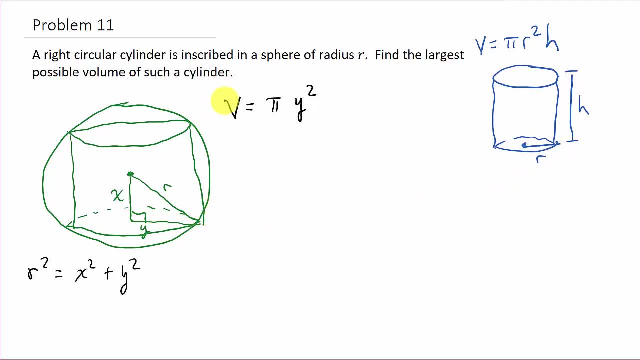 That's this distance here, And now times the height, So the height is 2x. Okay, This cylinder. see, if I go from here to here, that's x, And then if I continue on up to here, that's another x. 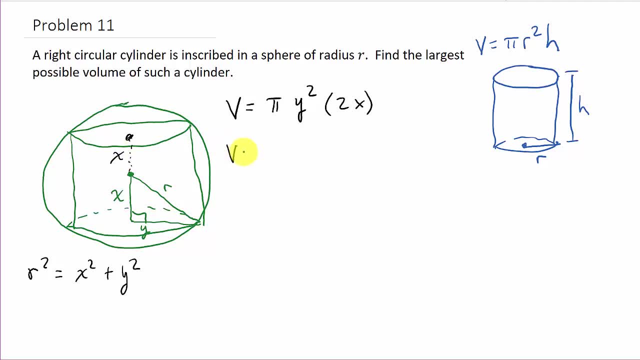 So that would give us 2x. So we get: the volume is 2 pi. Okay, So that's x times y squared. Just rearrange the terms. That's all I did. All right, So now what we're going to have to do is we're going to have to take the derivative. 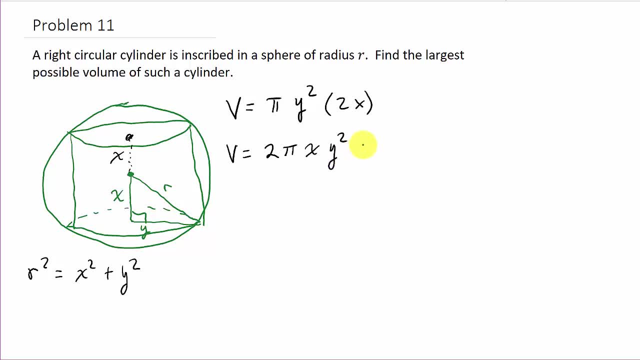 of this thing. Well, but what I'm going to do first is get everything in terms of one variable. Well, I'll get everything in terms of x. Okay, So if I take this and I subtract the x squared to both sides, I end up with y squared. 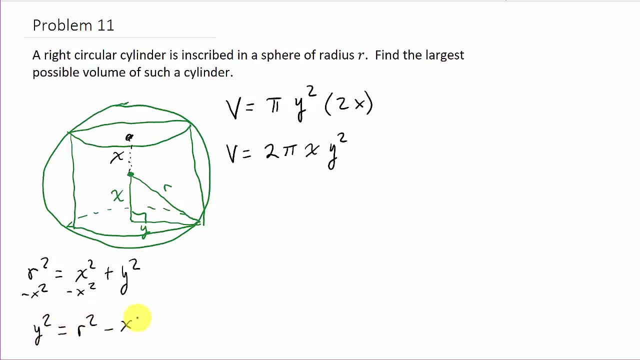 I end up with: y squared is equal to r squared minus x squared. So I can take this r squared minus x squared and replace y squared with it. See, I've got exactly what y squared is. So that gives me the volume is 2 pi times x, times r squared minus x squared. 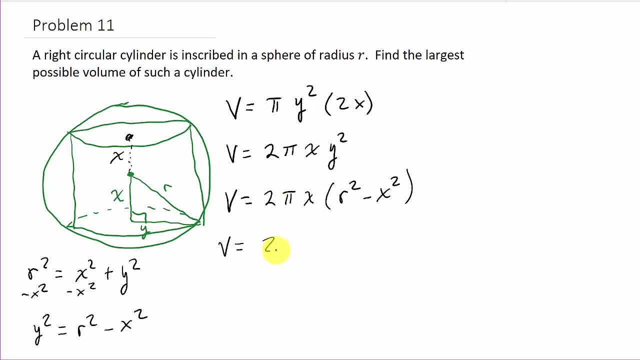 And then I'll distribute. So I get the volume is 2 pi x- Okay. So I get the volume is 2 pi x r squared, minus 2 pi x cubed. Okay, All right. So now I'm ready to take the derivative. 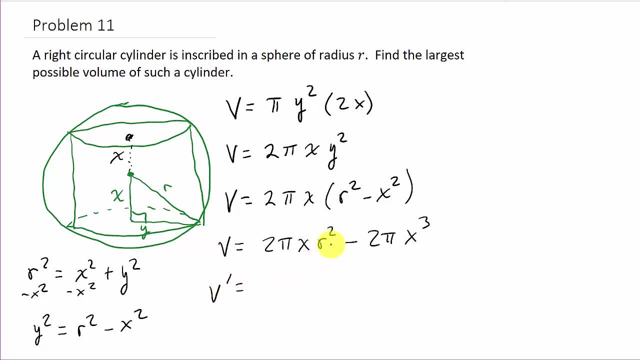 So the derivative is equal to what 2 pi r squared. Now, remember, x is our variable. We're taking the derivative with respect to x or we treat like a constant term. Okay, And that's minus, And then the 3 comes down. 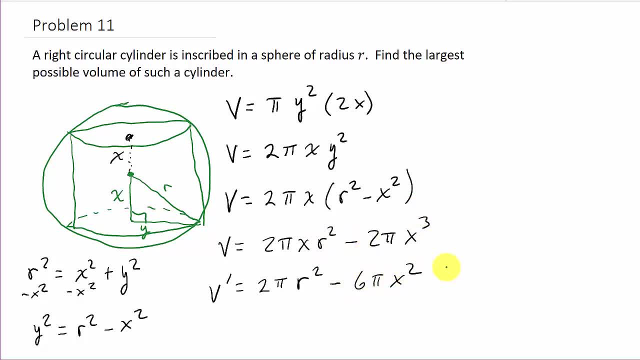 6 pi subtract 1 x squared. All right, So now what we have to do is set this equal to 0.. Okay, And solve for x. So I have 2 pi r squared minus 6 pi x squared equals 0.. 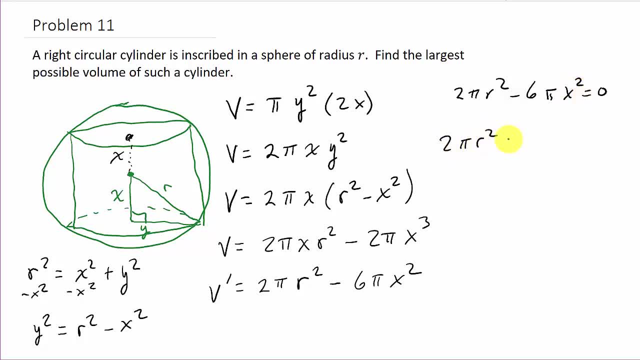 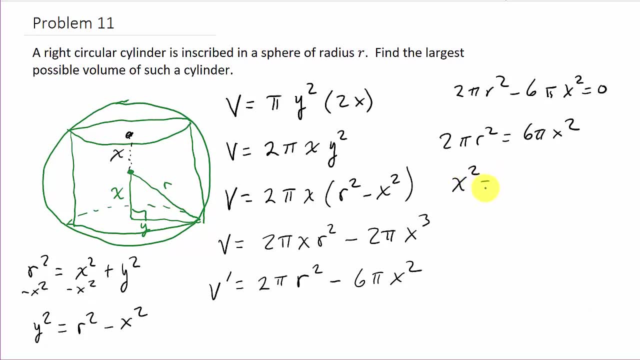 So that's going to be 2 pi r squared equals 6 pi x squared. Okay, And so I get: x squared is equal to: Now. I divide both sides by 6 pi. Okay, Now they don't look like it, but that's pi. 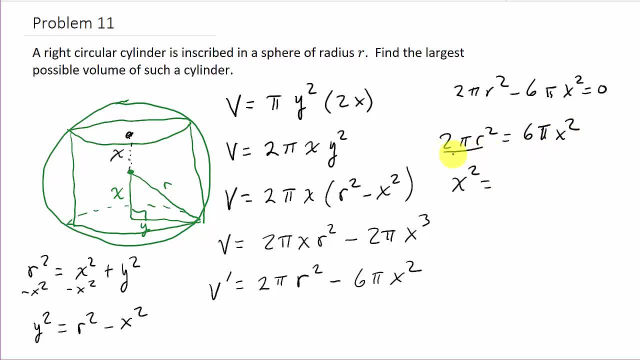 Okay, And so if I divide both sides by 6 pi, the pi's cancel and I'm left with r squared over 3.. And so I get: x is equal to r over the square root of 3.. Okay, All right. 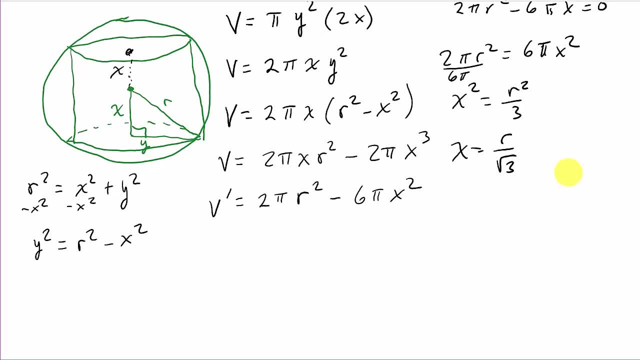 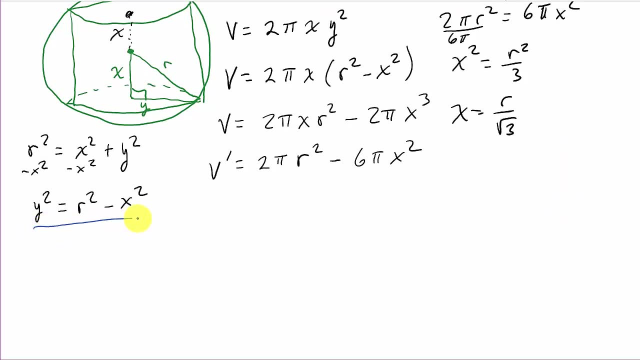 So there's x. Well, now we need to know what y is. Okay. Well, from this right here, we know that y is equal to the square root of r squared minus x squared. Okay, All right, So I can get. y is equal to the square root of r squared minus r over the square root of 3 squared. 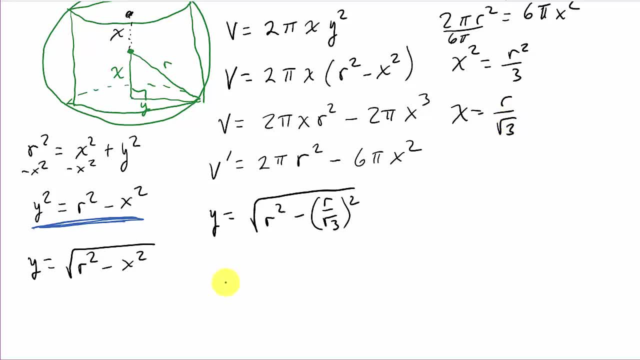 Plug that in for x, And so that's going to give me the square root of r squared minus r squared over 3 when I square that, And so y is equal to, So y is equal to the square root. Now when I combine those two, I get a common denominator of 3.. 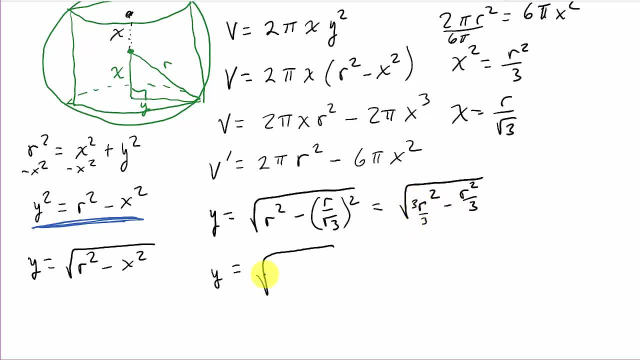 So that would be 3 and I would have to multiply by 3 here. So that's 2r squared over 3, which is equal to the square root of 2 thirds, and then the square root of r squared is just r. 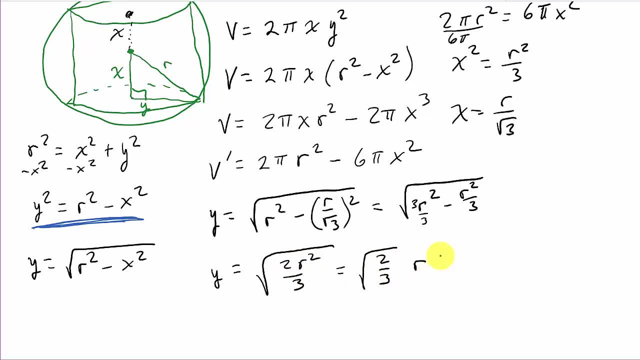 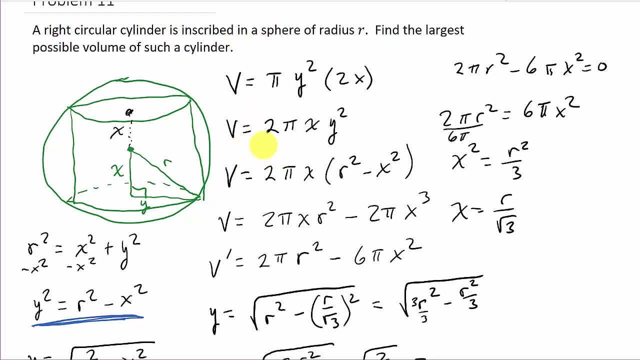 And so that's y. Okay, Now I have y. Now, remember, we want to find the largest possible volume, Okay, So what's the volume? Well, remember, this is our volume here. Okay, So we've got to take the x and what we got for y and plug it into here. 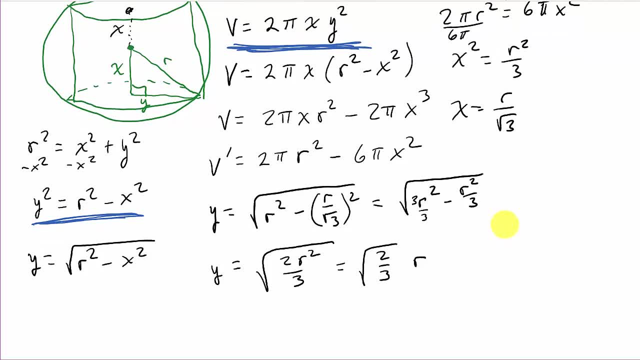 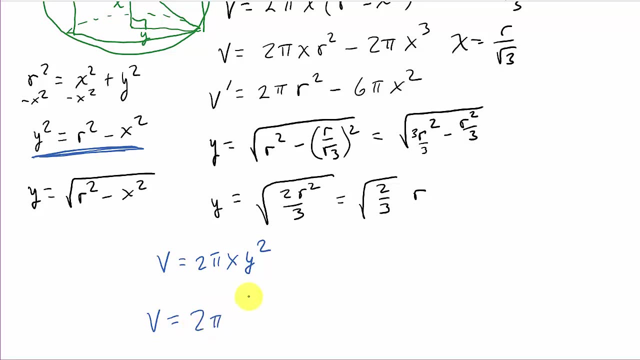 Okay, So let me write that volume down here. So the volume is 2 pi x- y squared. Alright, So the maximum volume would be 2 pi times x, which is this times r over the square root of 3 times y squared. 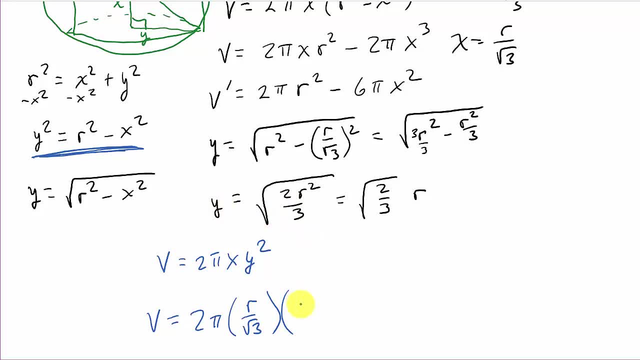 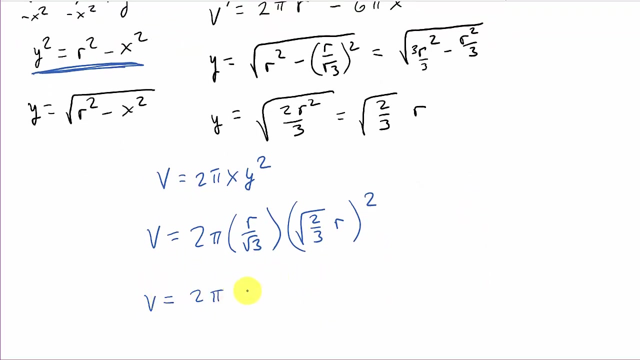 So that's going to be the square root of 2 over 3 times r squared. Okay, So let's see We get. volume is 2 pi r over the square root of 3 times 2 pi. Okay, So that's going to be 2 pi r over the square root of 3 times 2 thirds r squared. 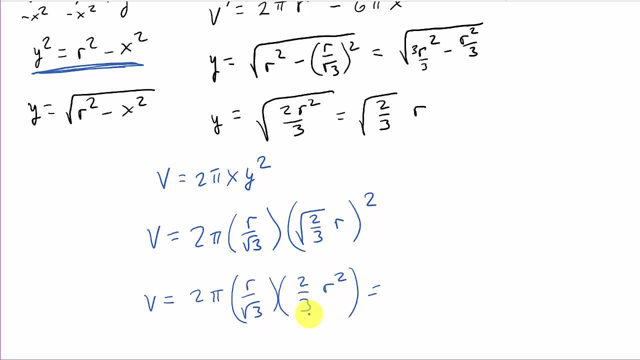 And then when we multiply this, let's see we get. see that's over 1.. So that's going to be 4 pi r cubed. Okay, See, r squared is r cubed. And then 2 times 2 is 4 times the pi. 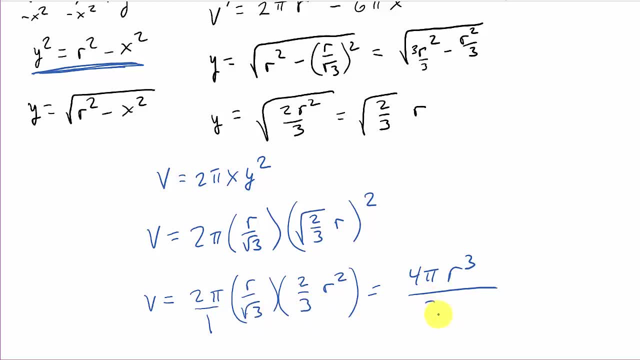 And then that's going to be over, then I'm going to multiply the denominators 3, square root of 3.. And whatever units this is in, it doesn't say but it would be cubic units, Okay, So there's our. there's the largest possible volume.